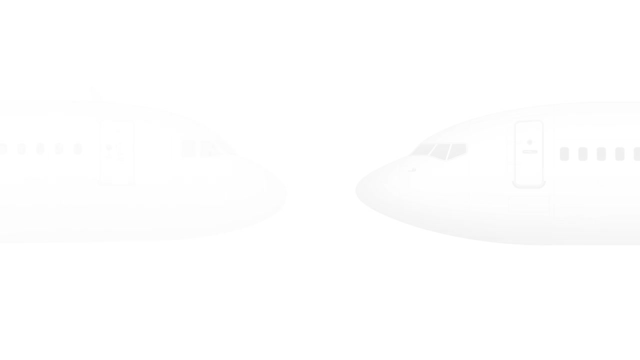 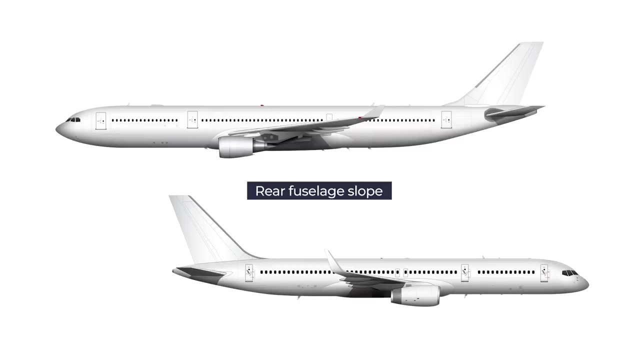 Boeing aircraft tend to have a sharper, more pointed nose. And, as a final generalization, consider the rear of the fuselage. On Airbus aircraft other than the A380 and A350, the fuselage continues straight to the APU exhaust. On Boeing aircraft it usually tapers downwards. 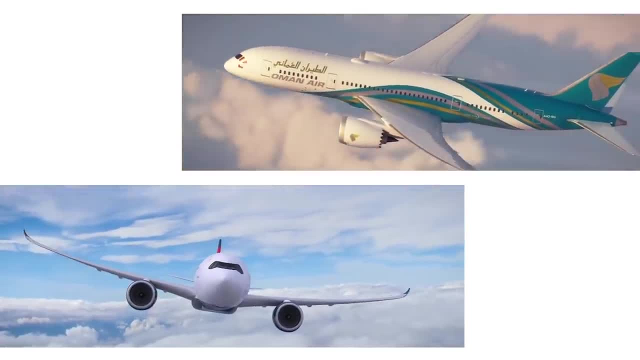 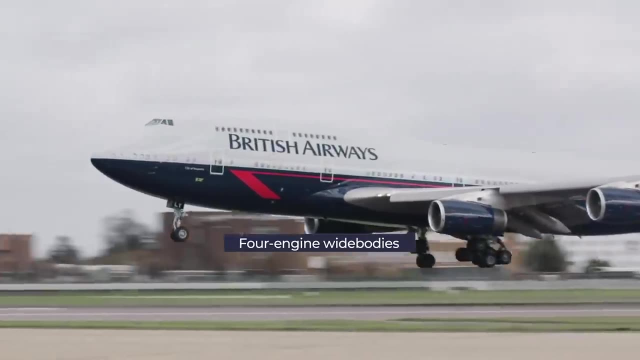 Now that some broad generalizations are out of the way, let's drill down into the specifics of each of them. aircraft: We'll start with the simplest to identify: four-engined widebodies. There are only three four-engine aircraft types in common: commercial service. 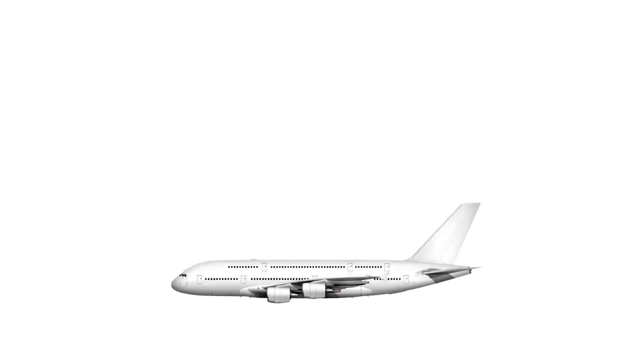 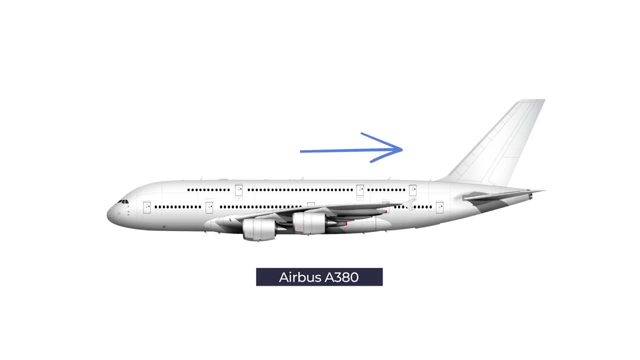 The A380,, of course, is the newest and quite easy to identify with its two full-length passenger decks. A straight line from the cockpit to the tail, with two rows of windows, should give it away If you're still onshore. the A380 is the only quadjet to have tip-fenced-style winglets. 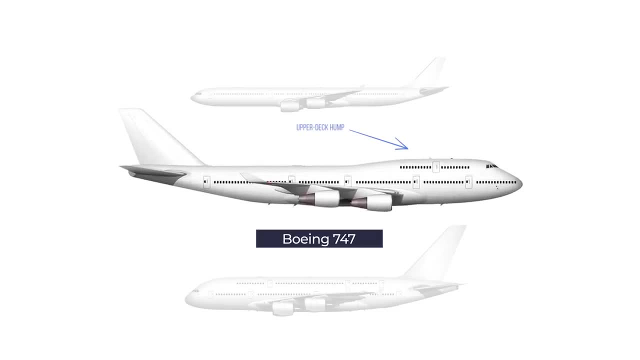 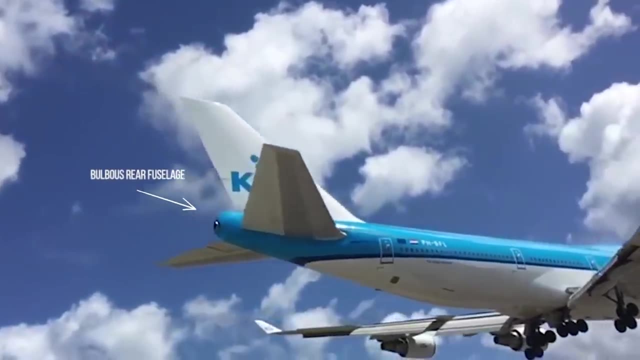 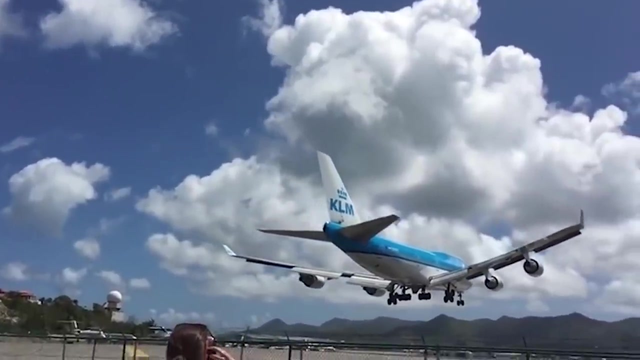 Likewise, the 747 needs little introduction or guidance with its iconic partial second-deck hump From behind. its bulbous rear fuselage is also quite distinctive. But then there are differences between 747 variants With multiple generations of 747s. let's look at the two latest: the Dash 400 and the Dash 8.. While the older Dash 400 has winglets and four conventional-looking engines, the newer Dash 8 is characterized as a more modern-looking engine. The newer Dash 8 has winglets and four conventional-looking engines. 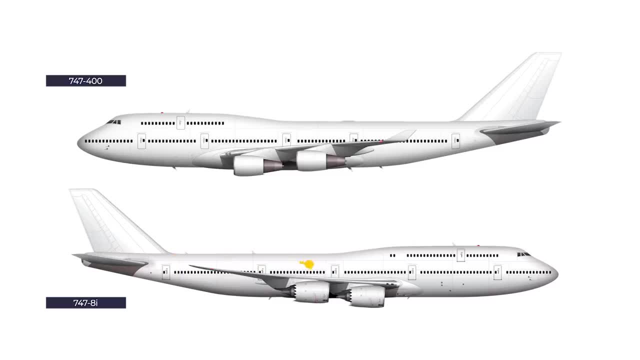 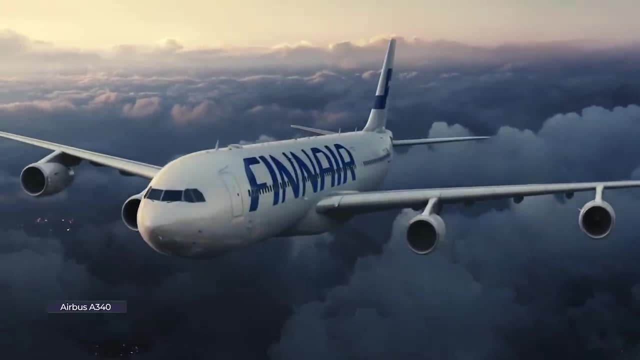 The newer Dash 8 has winglets and four conventional-looking engines. The newer Dash 8 has a longer upper deck, a lack of winglets and engines with chevrons. The other four-engine aircraft in regular commercial service is the Airbus A340.. 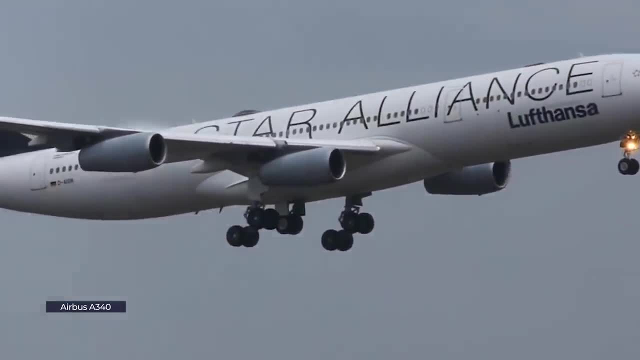 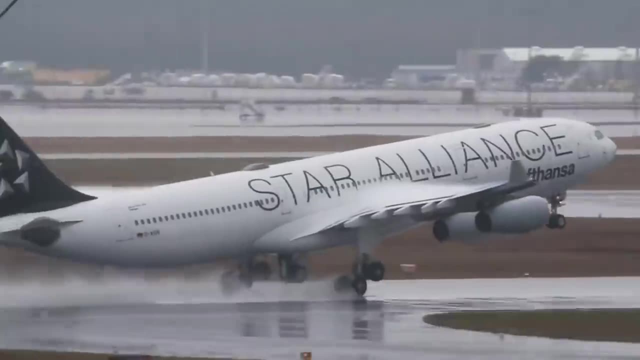 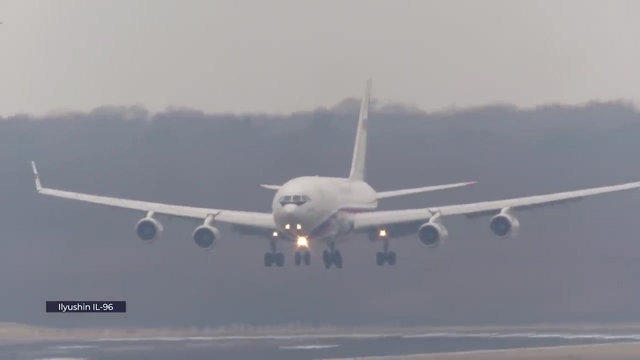 If you're outside of Russia and looking at a four-engine widebody with only one row of windows going from the cockpit to the tail, it's almost certainly the A340.. With our focus on Airbus and Boeing jets, we'll exclude the Russian IL-96 from this video, which has higher and more vertical. 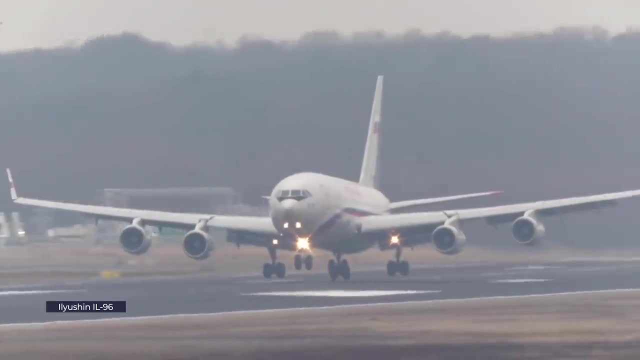 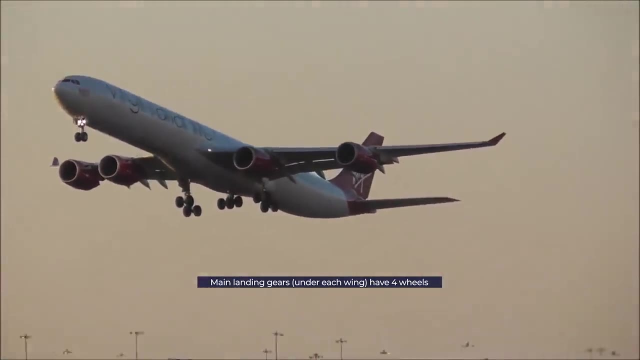 winglets, and the Airbus A340 is the A340.. The Airbus A340 is the A340.. The Airbus A340 is the A340.. And a more bulbous shape than the long and skinny A340.. The A340 has four-wheel main landing gears. under each wing The additional central landing gear. 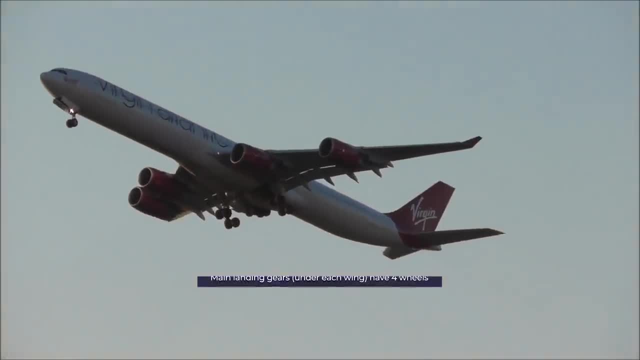 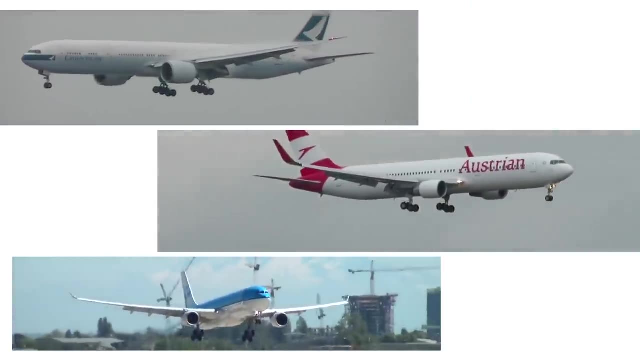 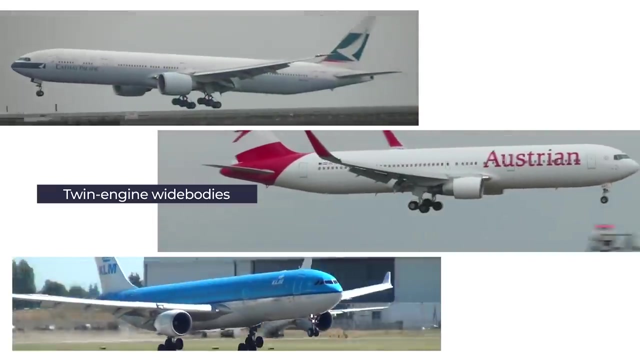 has two wheels on the A340-200 and 300, and four wheels on the A340-500 and 600.. Moving on identification gets harder with twin-engine aircraft. Again, we'll proceed through each aircraft family separately, but remember there are characteristics. 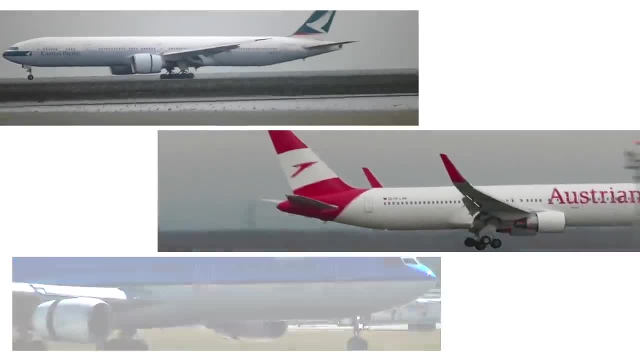 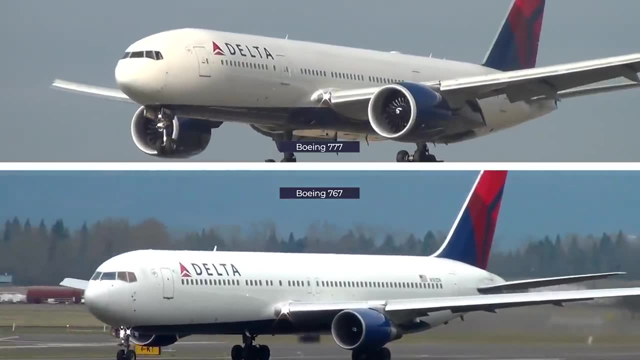 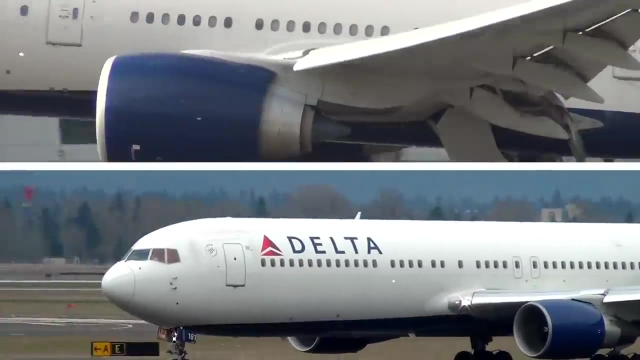 in either aircraft types. that can help by elimination. The Boeing 767 and 777 can be hard to distinguish from a distance. They both have the typical features of Boeing style, such as their windows and tails. However, the 767 is much shorter. In fact, the most common 767-300 variant is 55 meters long. 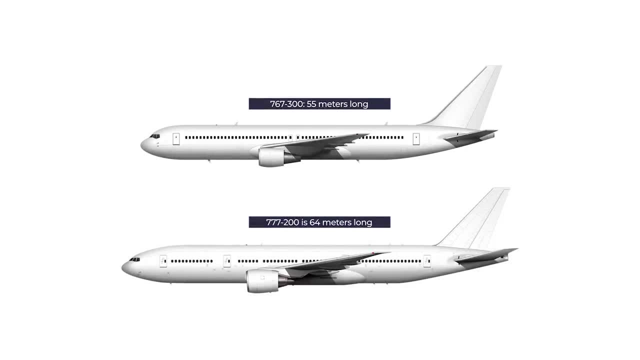 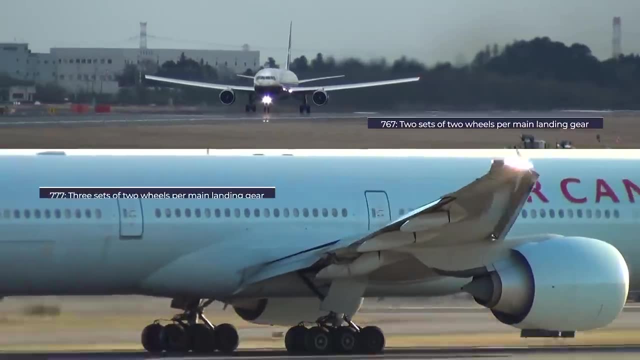 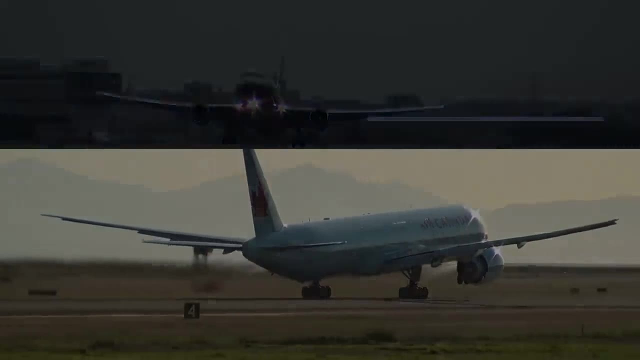 compared to nearly 64 meters long for the 777-200.. The wheel arrangement is also different for each type. The 767 has a two-wheel main landing gear, whereas the 777 has three wheels. The 767 can sometimes, but not always, be differentiated by its winglets. 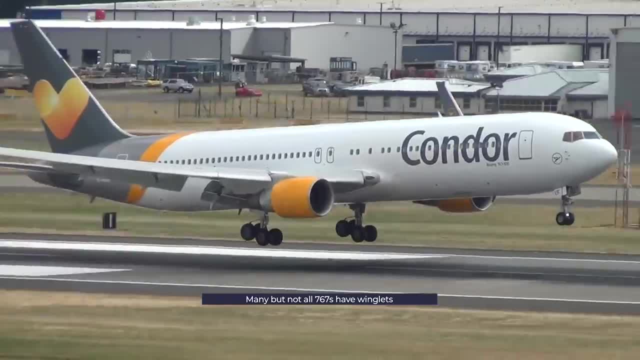 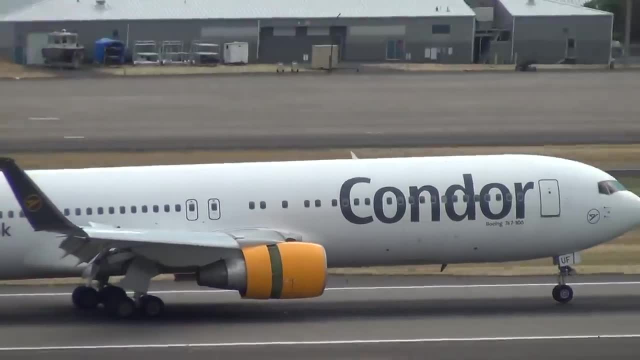 It's the only wide-body aircraft to have winglets that curve up with an L-shape. Not all 767s have these, however, which make it an unreliable feature for identification. Purely going by size, it can be easy to confuse the 767 with the A330.. 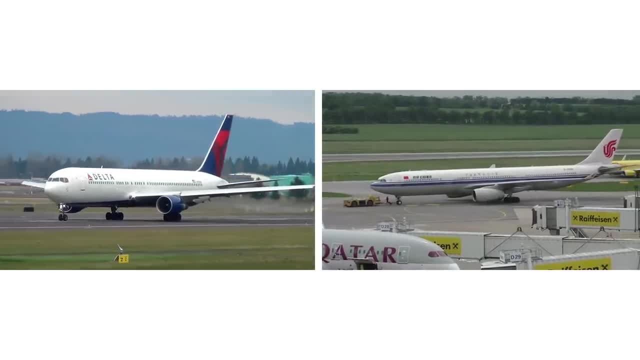 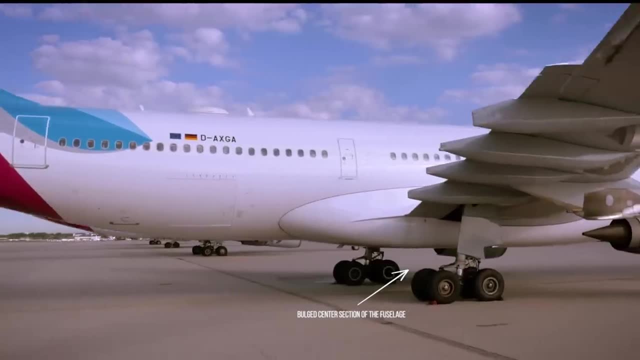 Apart from the standard Boeing and Airbus differences, there are also key differences underneath the aircraft. The A330 has a bulged center section of the fuselage between the wings. The main landing gear wheels also slope to the rear when extended On the 767,. 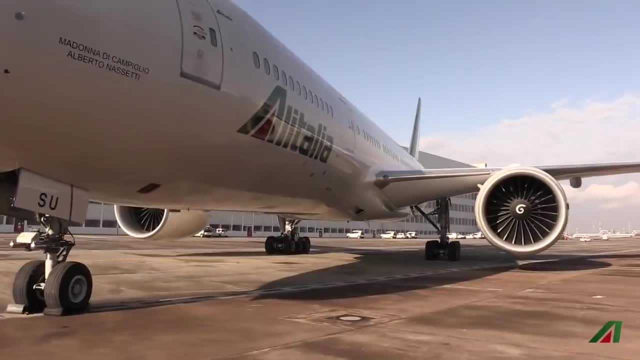 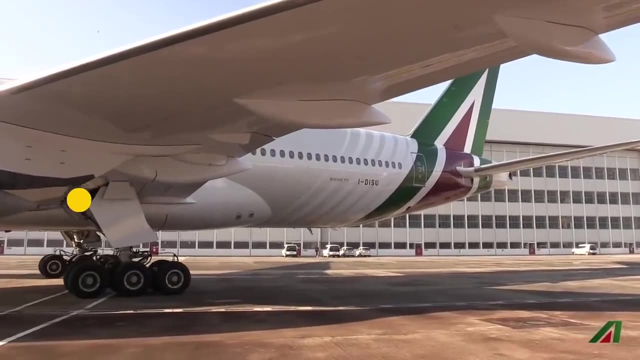 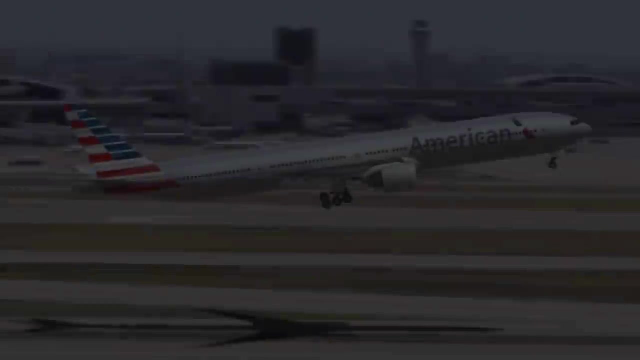 they slope to the front. Ultimately, the two most reliable ways to identify the 777 are its main landing gear wheels and its rear exhaust. It has three pairs of wheels on each gear. Of all twin widebodies, only the 777 and the A350-1000 have this. 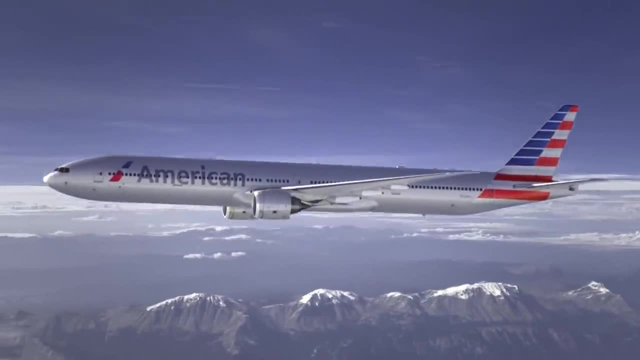 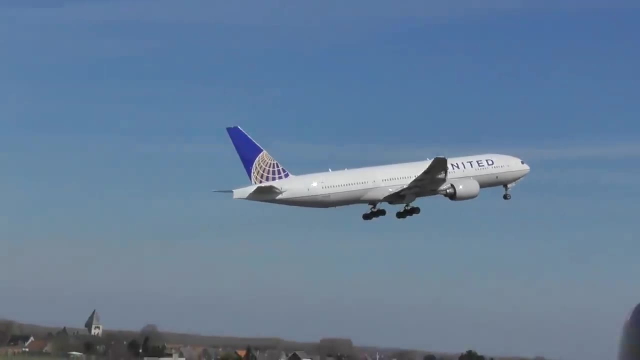 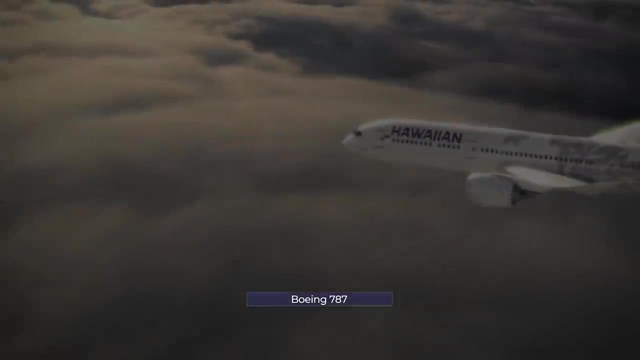 The 777's distinctive APU rear exhaust design is bladed or sawn in appearance rather than conical as seen on other twin engine jets. This is a great way to always tell the 777 apart. The 787 is an easier aircraft to identify, with several distinguishing features. It has a distinctive 4-pan 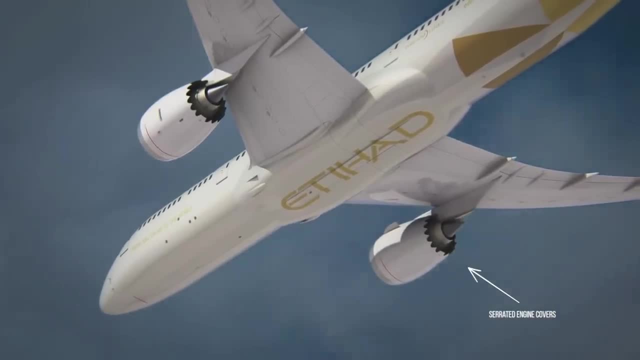 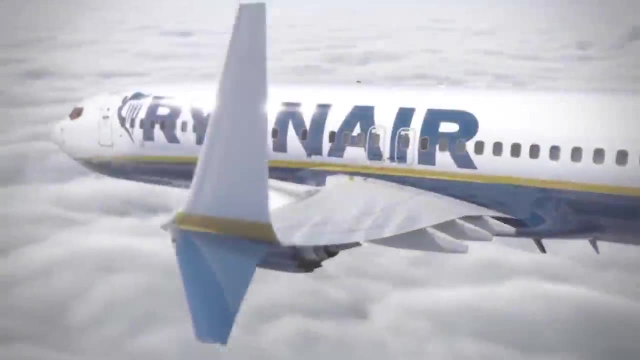 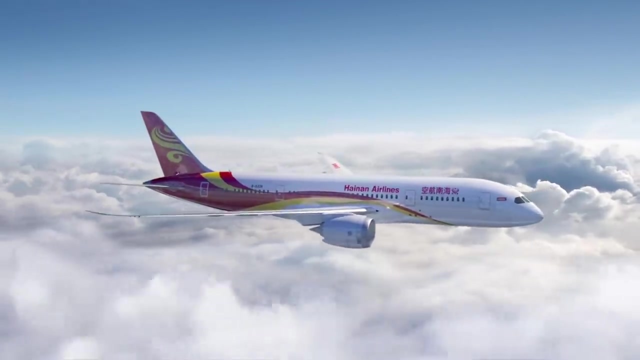 screen and is the only wide-body twin with serrated nacelles housing the engines. The 747-8 has four of these engines, while the narrow-body 737 MAX has two. The 787 also has a very distinctive smooth nose design. This is quite different from the 767 and 777, almost blending seamlessly into. 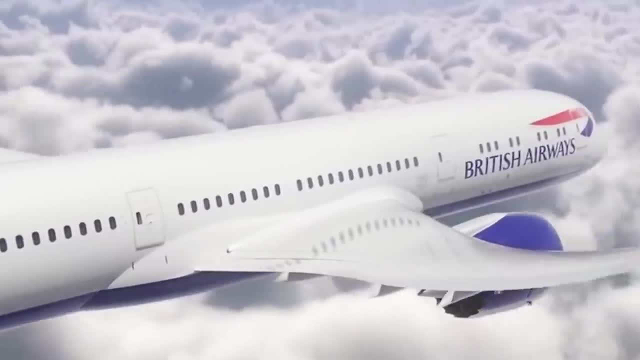 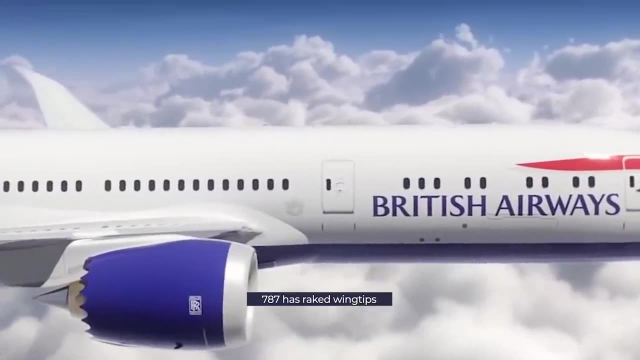 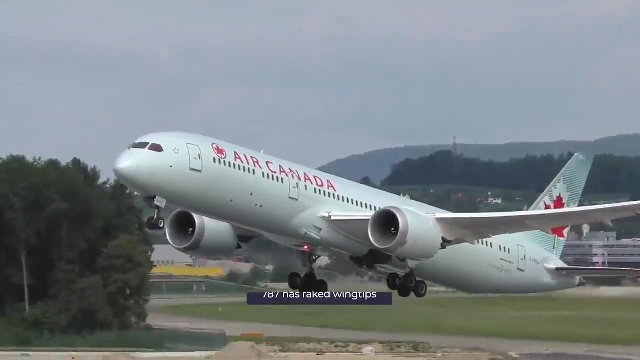 the cockpit windows. With its raked wingtips, the 787 does not have winglets compared to the similar-sized A350.. In flight, the 787's flexible wings are easily distinguished. During take-off and landing, these seem to flex upward- a very unique feature. 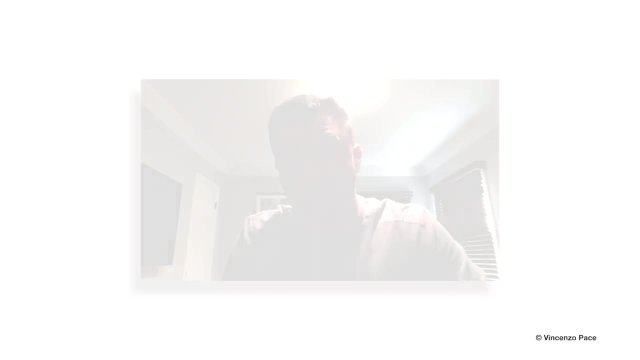 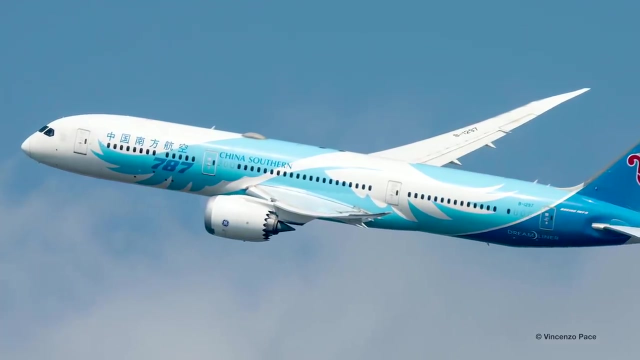 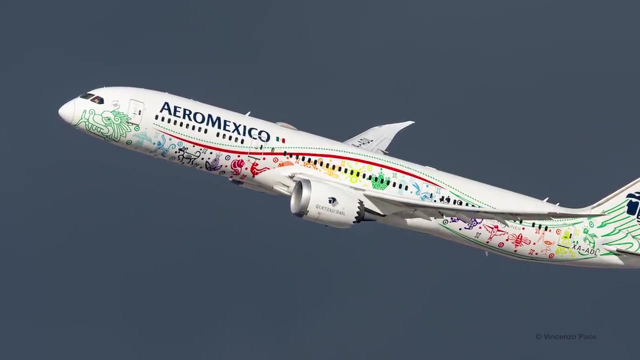 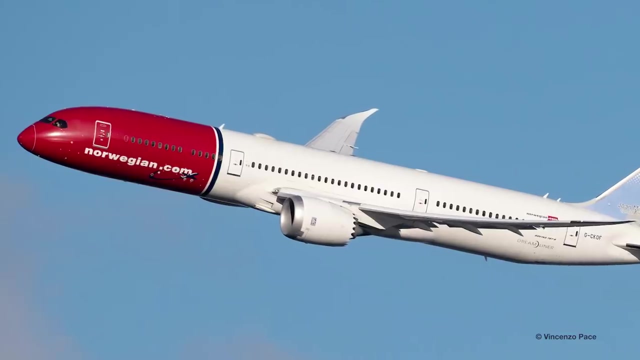 One of my favorite shots that I've ever taken out of JFK is a banking shot which slows a heavy flex of the 787, which is a very unique characteristic, a very signature characteristic of the Dreamliner and pretty much 90% of the time when a Dreamliner leaves on that departure it will always give a nice performance. 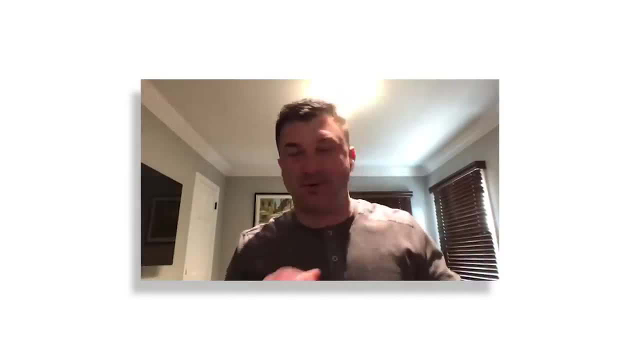 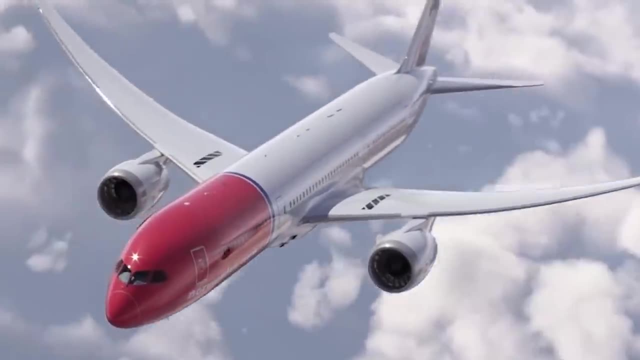 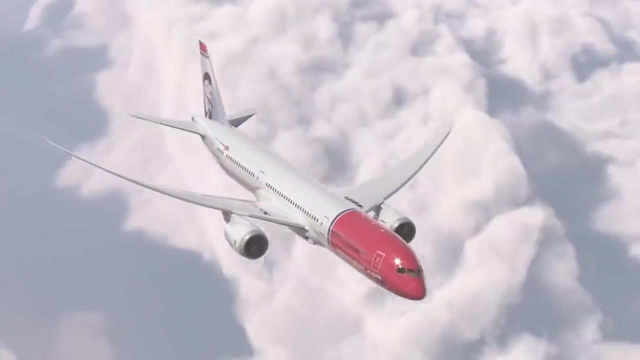 of a very fine wing flex, And also on the Dreamliner you have the serrated engines, which is a clear characteristic of a Boeing aircraft, the swooping nose- a very modern nose- and cockpit in the window. So the Dreamliner has a very unique signature. from a shot taken: 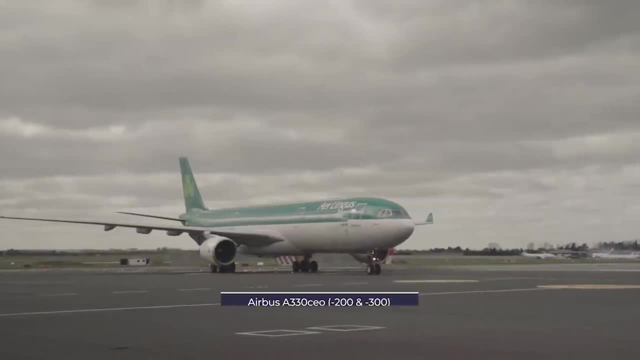 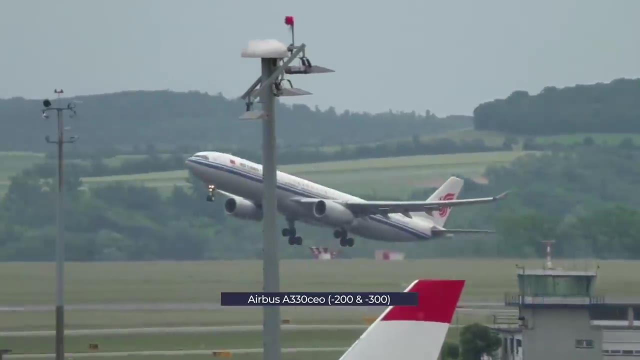 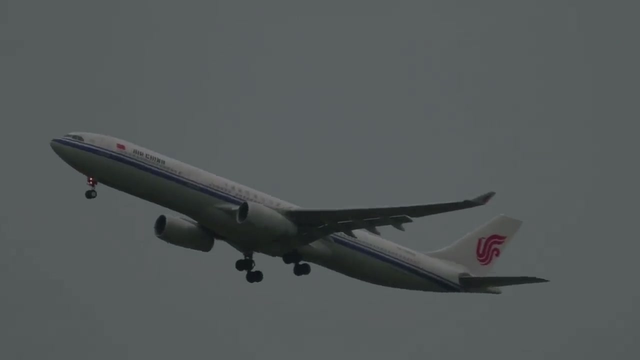 on that approach. The older Airbus A330s are distinguished by their traditional Airbus cockpit windows and angular winglets. These winglets aren't found on any other twin-engined widebodies, although the 747-400 does have something similar. Telling the Neo variants apart from the earlier ones is quite straightforward. 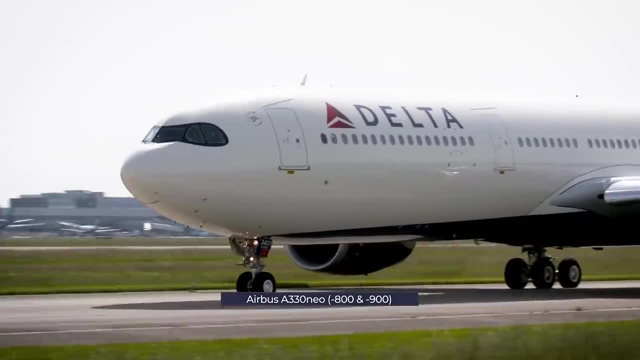 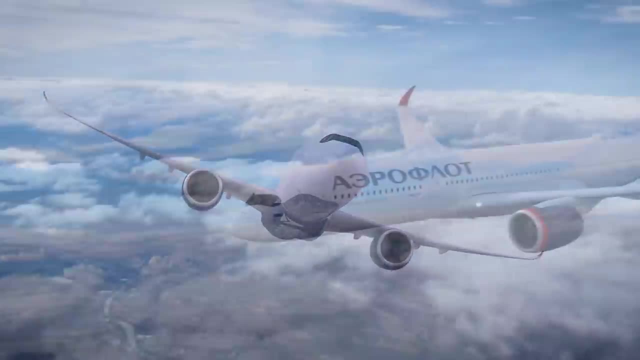 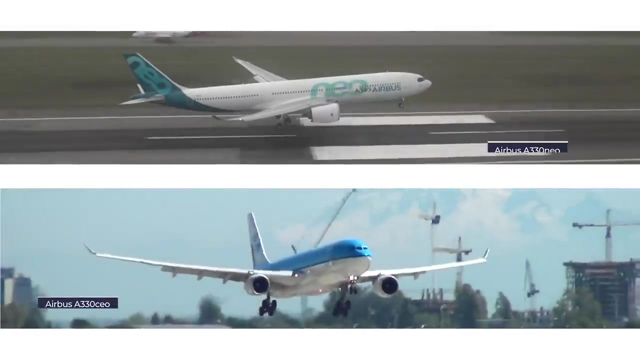 The A330-800 and Dash 900 have a different window design with black edges, sometimes referred to as raccoon style. These are similar to those on the A350.. The A330 Neos also have different wingtips. The A330-200 and Dash 300 have straighter angular. 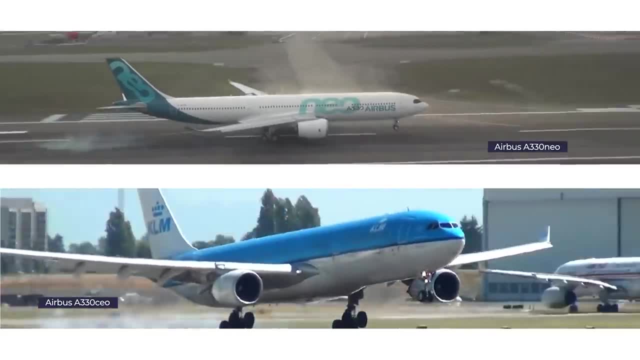 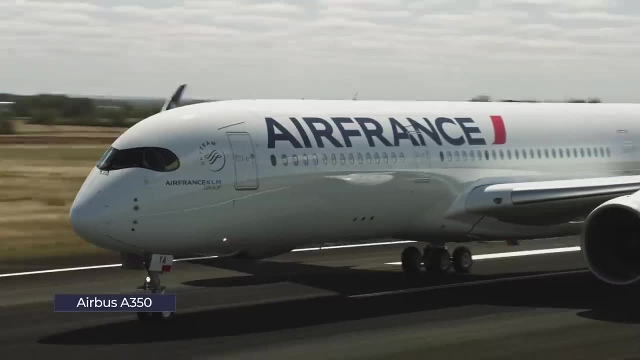 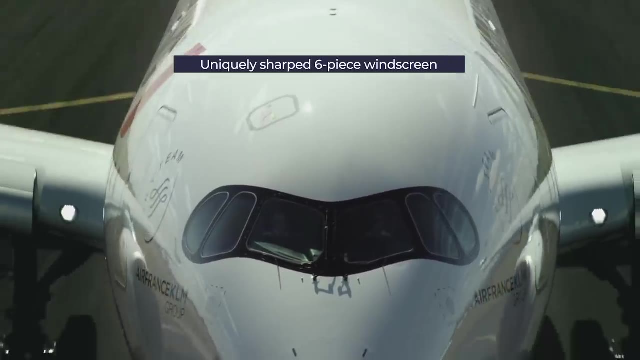 winglets, whereas the Neo models have smooth blended sharklets. The A350 is another easy-to-identify aircraft with a couple of main distinguishing features. It has a unique six-piece cockpit windscreen. This has side windows with curved edges and a black 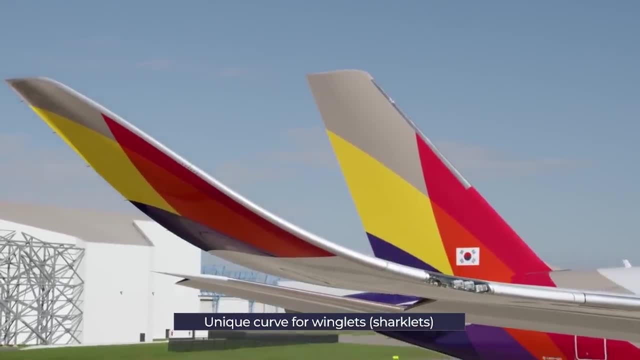 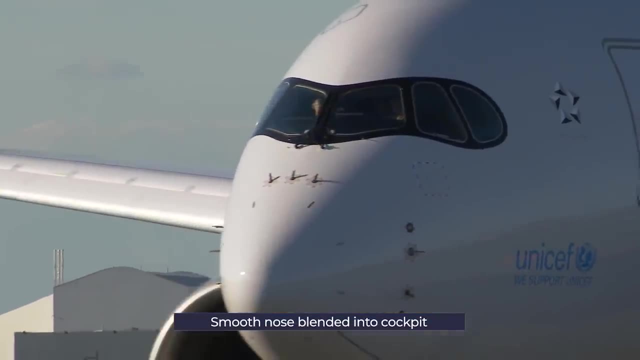 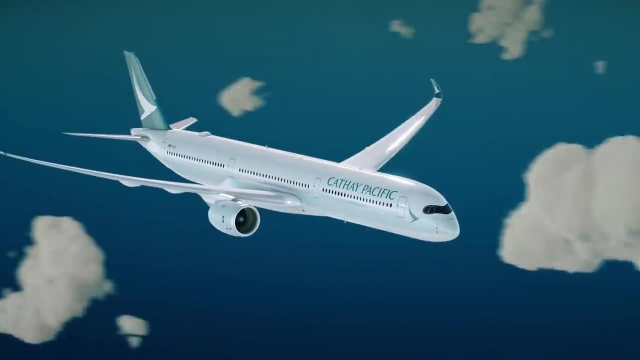 frame design. The A350 have fairly distinctive curved winglets And, like the 787,, it has a smooth nose design, unique amongst other Airbus aircraft. The thing that really makes and can really tell you what a 350 is is it's commonly nicknamed. 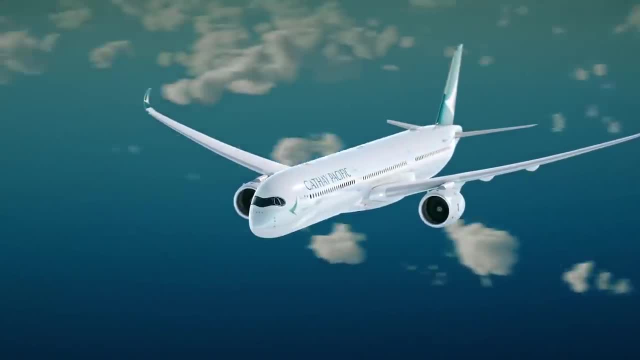 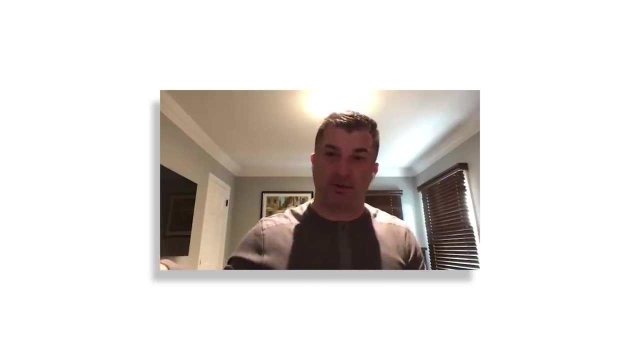 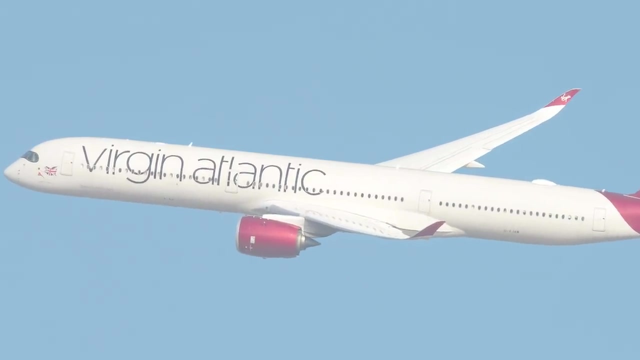 it's called a raccoon. because of its cockpit windows and its nose It gives the impression of looking like a raccoon. but also its beautiful winglets. It's really beautiful to see. You can't imagine the winglet on the opposite side of the plane to really show up on that. 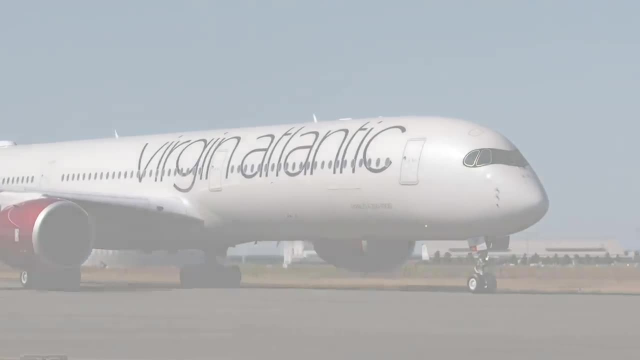 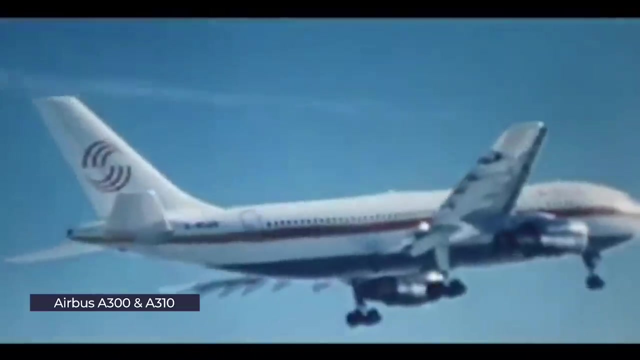 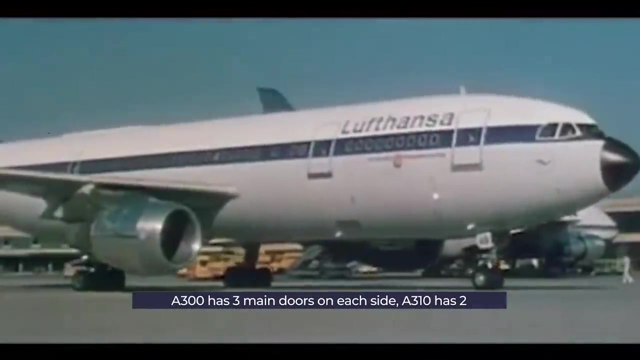 banking shot Moving from Airbus's newest wide body to its oldest. the A300 and the A310 have a flat central fuselage, not bulged as on the A330.. The A300 has three main doors on each side and one exit to the rear of the wing, whereas the shorter A310 only has two main doors. Of Airbus' wide-body jets, the A300, E-Bus A330, and the A310 have one exit, to the rear of the wing. The A300 has a wide-body fuselage only having one door on both sides, while the A310 has two doors in the back. 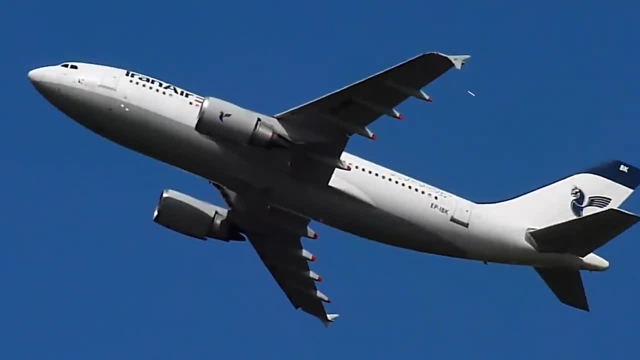 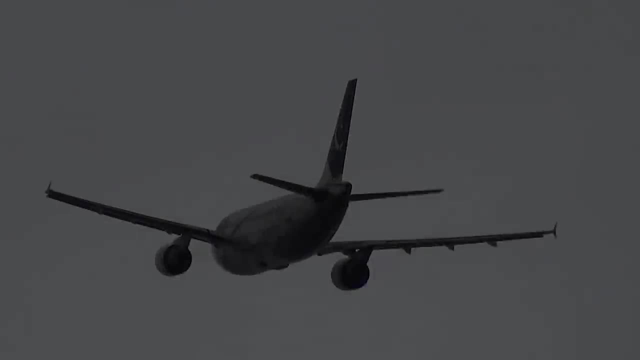 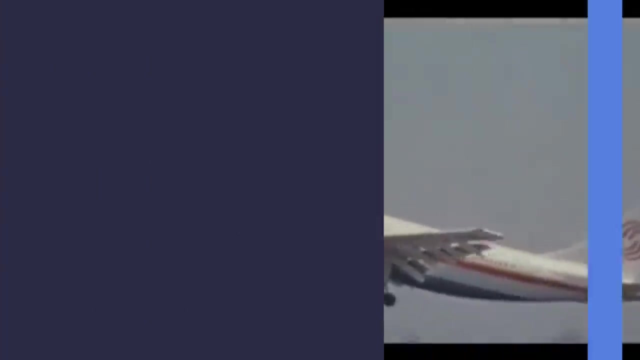 As well as wide-body jets. the A300 and A310 are the only twin-engined aircraft to have tip-fence-style winglets, which you'll also see on the A380.. Of course, to complicate things, these winglets aren't present on all A300s or A310s. 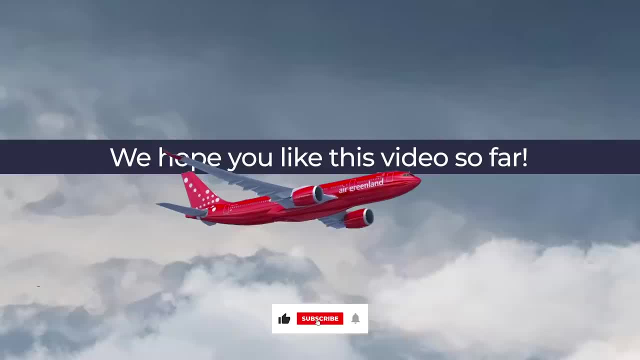 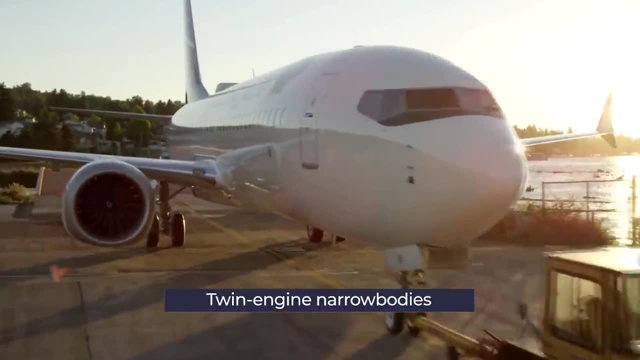 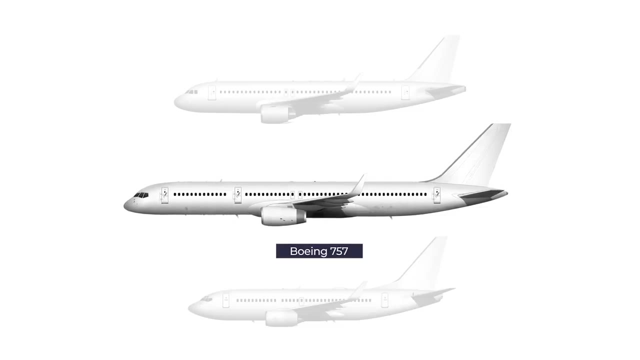 If you're liking this video so far, why not click subscribe and hit the like button? Oh, and be sure to click that notification bell too. Moving on to twin-engine narrowbodies: To distinguish the 757 narrowbody from the 737 or A320 family, look for the following: 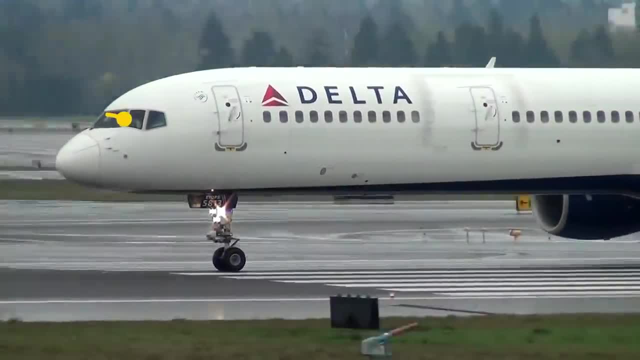 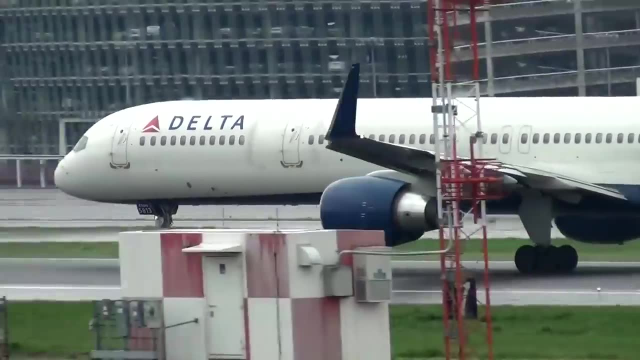 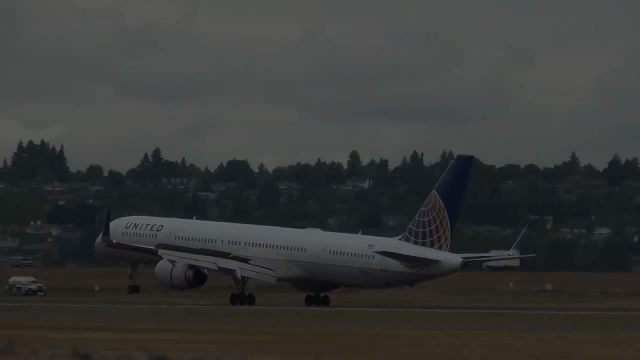 Boeing-style cockpit windows, A distinctive dolphin nose- like any nose differentiation- this takes practice- And a taller landing gear than the 737 or A320.. It also is missing the triangular section between the tail and the fuselage seen on the Boeing 737.. 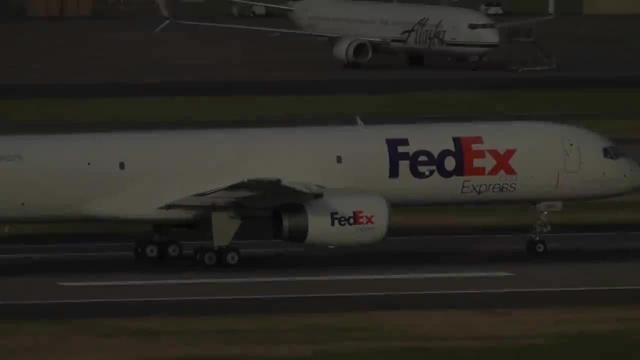 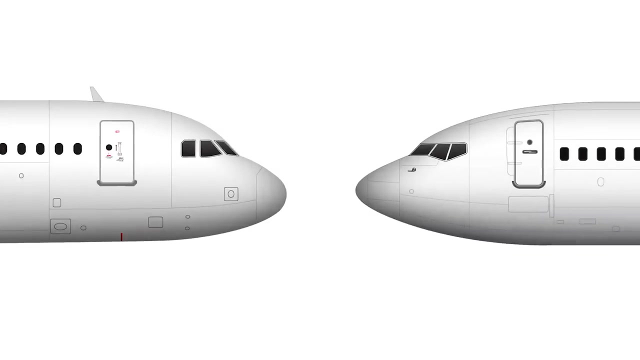 Some 757s have a tall blended winglet, But not all of them, which makes it an unreliable differentiator. Of course, most narrowbodies flying today are from the Boeing 737 and Airbus A320 family. To distinguish the two, you can rely on the Airbus vs Boeing window differences and the 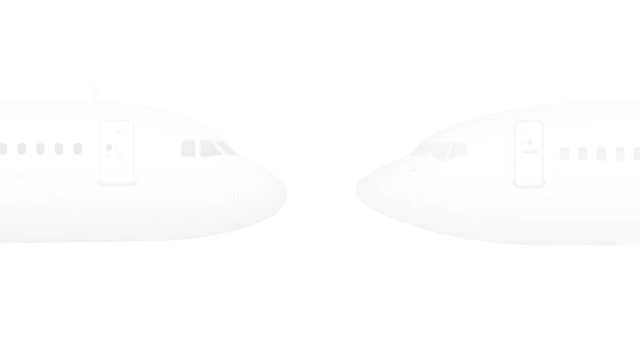 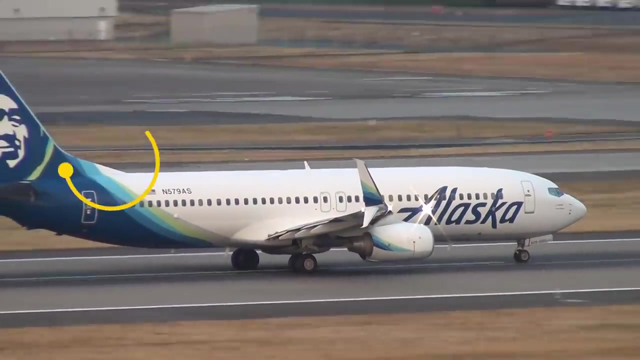 more pointed nose on the 737.. The 737 also adds two distinguishing features. It has a triangular, dorsal-like fin leading from the top of the fuselage to the tail, And it's also got a 3-way system. The fuselage is a two-way system. The fuselage is a two-way system And it's a two-way system. The fuselage is a two-way system. The fuselage is a two-way system, The fuselage is a two-way system And the fuselage is a two-way system. 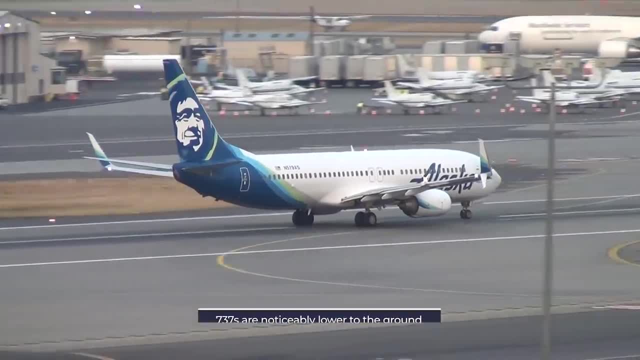 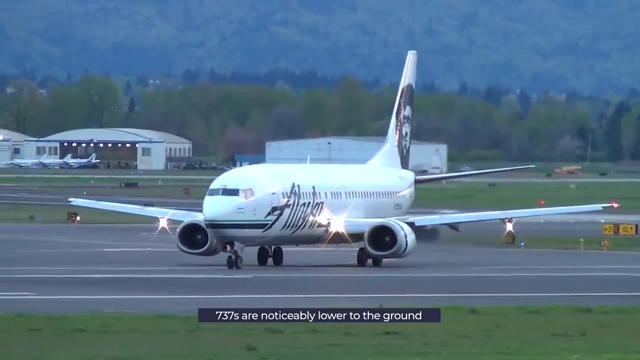 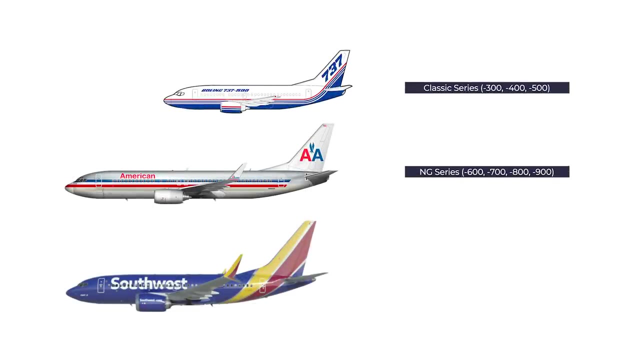 to the tail. Additionally, the 737s are lower to the ground, with most having engines with a flattened base. To distinguish different 737 variants, the following will help: The classic series does not have winglets. the next-generation series does. The 737 MAX is easily distinguished. 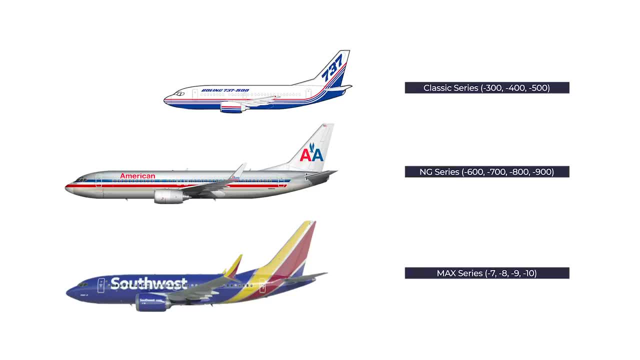 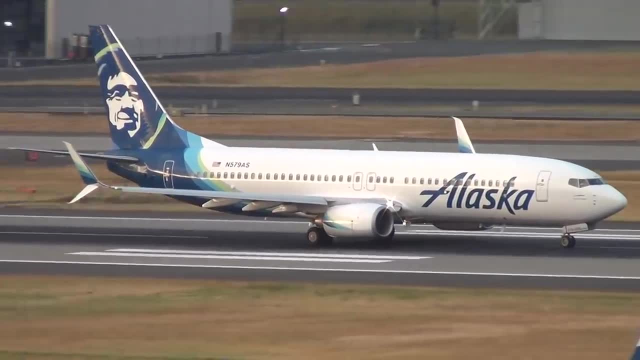 with a combination of serrated engine housings and larger split-scimitar winglets. Some 737 next-generation models have these split-scimitar winglets as well, but wouldn't have the serrated engine nacelles of the MAX family. 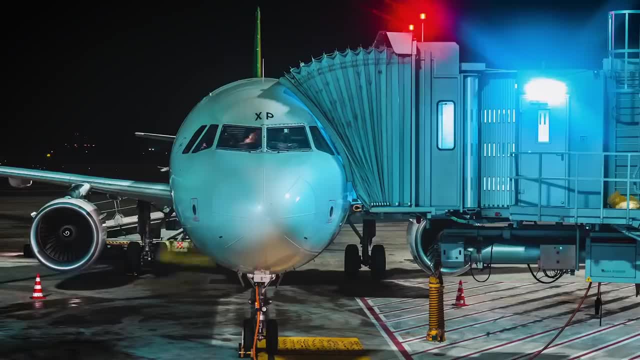 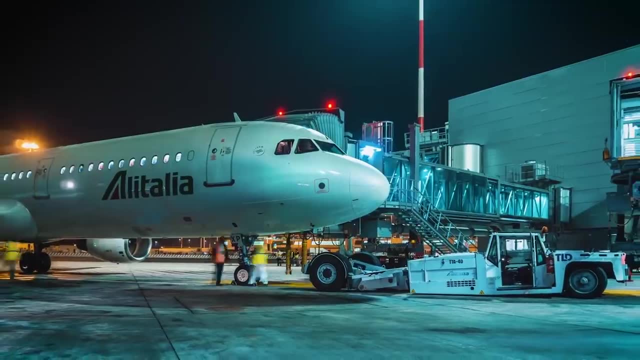 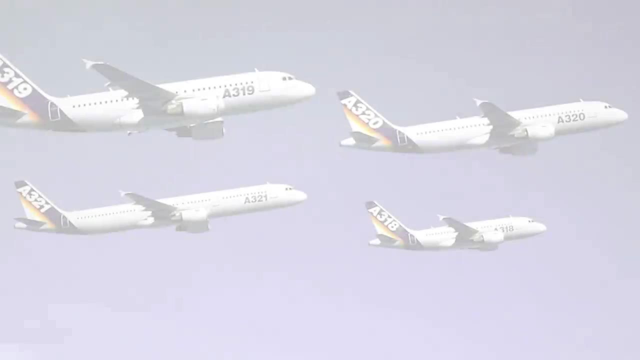 As with the Boeing 737s, the A320 is easily identified from the characteristic cockpit windscreens- straight rather than V-lower edge and notched corner And a more rounded nose. It also lacks the triangular dorsal fin section seen on the 737.. 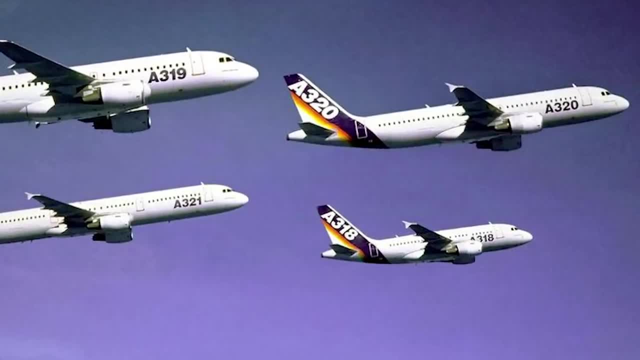 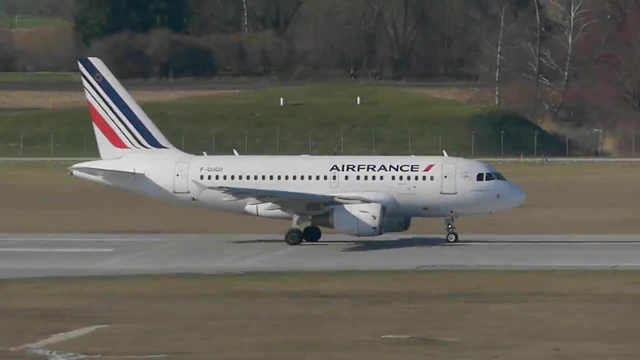 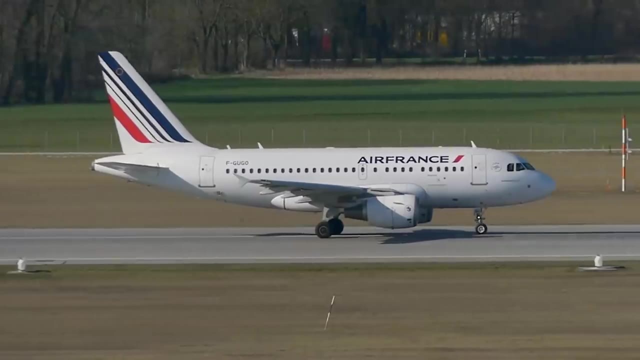 And again, the family members A380s and A730s do not have winglets. The A318,, A319,, A320,, A321, and NEO versions are best identified by their size. The A318 and A319 have one overwing exit door and two main doors To differentiate between. 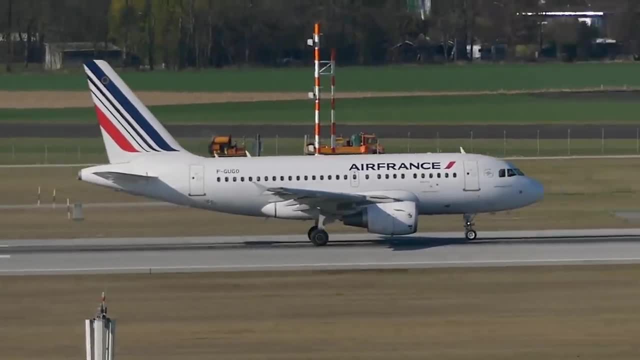 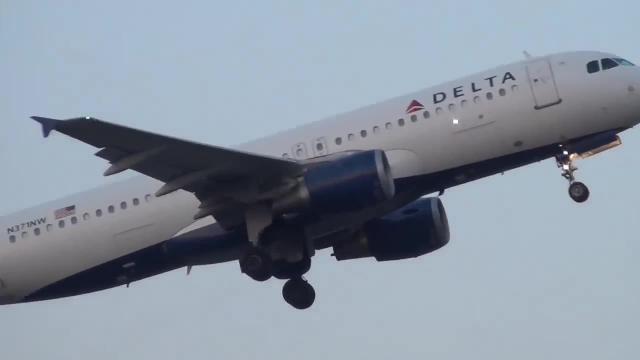 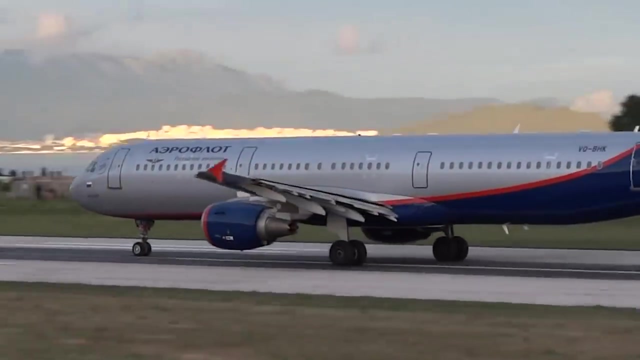 them. the A318 has 11 windows in front of the overwing exit. the A319 has 13.. The A320 has two overwing exit doors. Finally, the longest A321's wing is the A320.. The A321CO has four doors along the fuselage, not overwing. However, the A321LR has three. 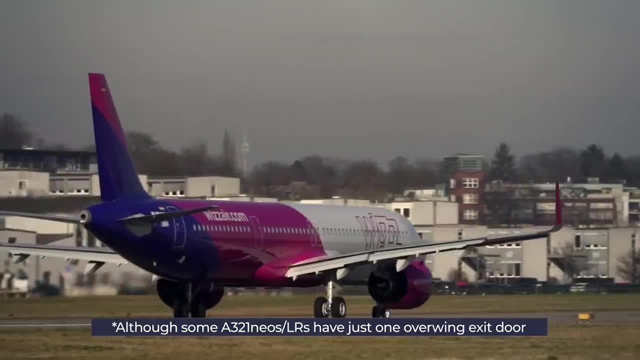 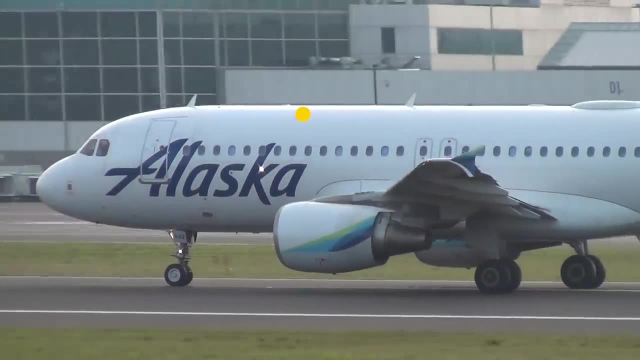 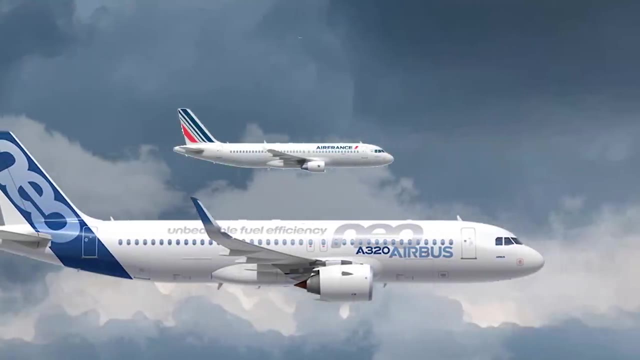 doors plus two smaller overwing exit doors. To identify the NEO variants, look at the wingtips and the engines. The A320CO will typically have tip-fence winglets, although some are retrofitted with a longer blended winglet. The NEO engines are larger than their CO counterparts. They also have extensions. 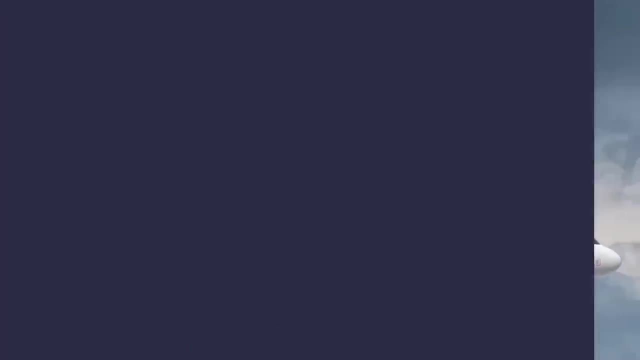 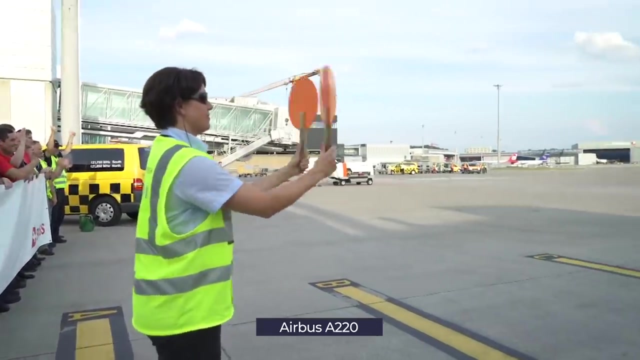 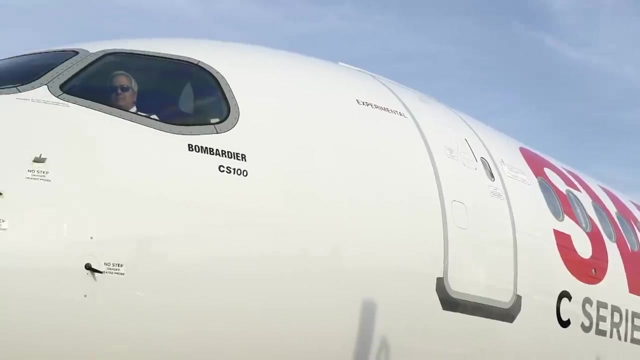 visible at the rear of the housing. The A220 was, of course, developed as the Bombardier C-Series. As such, it looks quite different from other Airbus narrowbodies. as it's effectively been adopted into the Airbus family, It is easily identified by its much sleeker, pointed nose and different-style four-screen windshield.